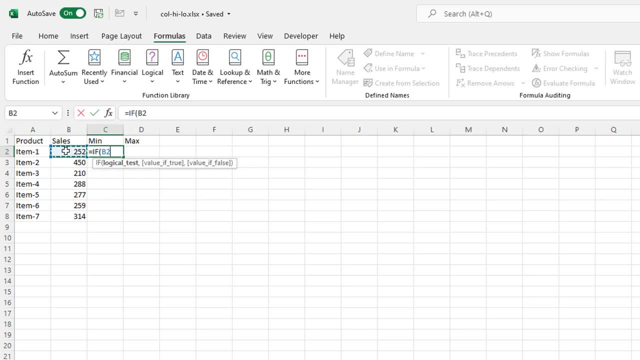 So it's going to say: if this cell equals the minimum of this range here and press F4 to lock that in, because then when I copy it down I don't want those to change. If that is true, then give me back this cell. If not, give me an NA- Close parentheses. 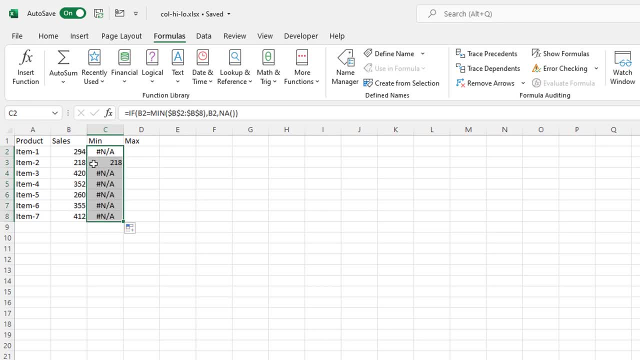 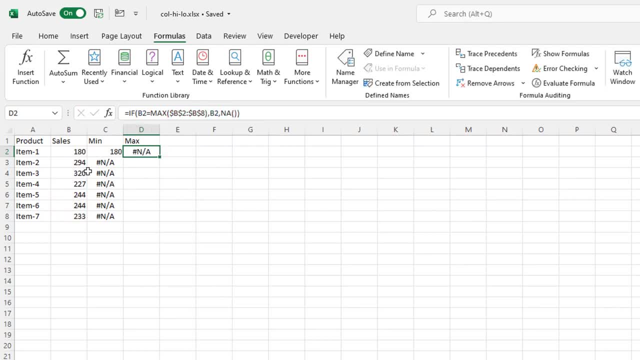 And if B2 equals B2 to B8, I want this to be the max M A, X. If it then bring back B2, that's right. Control enter And it stays in that cell. Double click the fill handle. 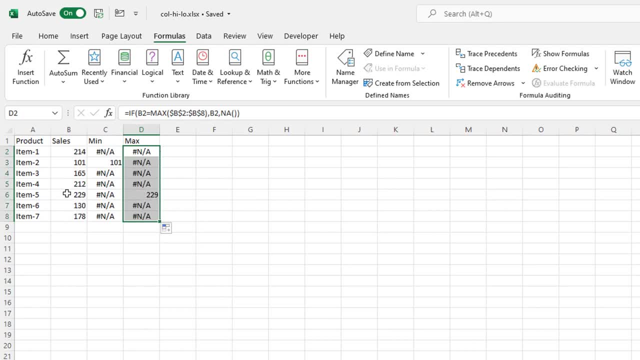 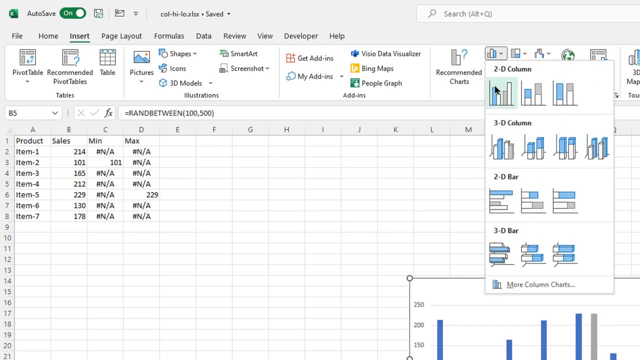 bring that down. 229 is the maximum here And 101 is the minimum there, So that's perfect. Now I need to bring this into a chart. Go to insert. Let's go insert a column chart And we can see that we've got our data here. Let's get rid of these grid lines. 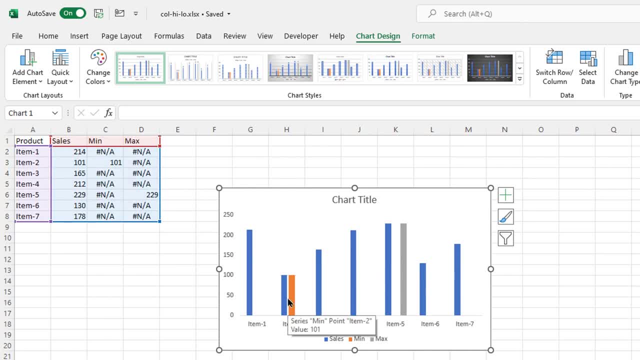 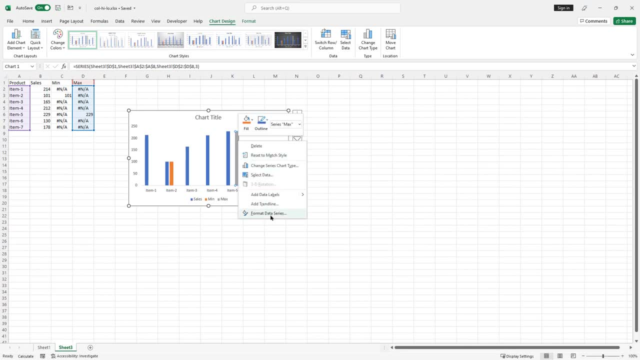 I want to do all the visual design before I put these two columns together, before I mush them together. So let's take care of that first. So the high one, let's make that one green And let's right click format data series. I want to format that data series. Make sure the S 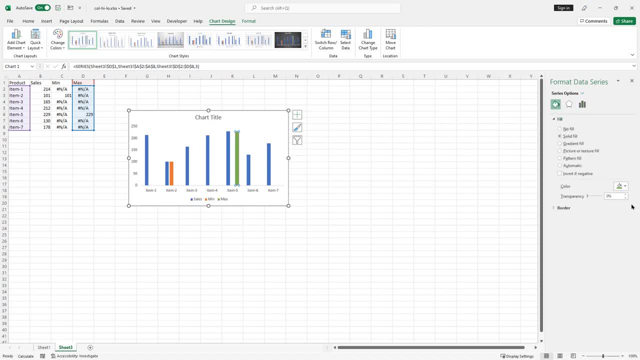 is there And under the paint, let's make that one green. Do the same thing for this orange one. Select on that. Format data series S: Let's make this one orange. And then for the rest here format data series, let's make that one gray. So that's nice and gray. 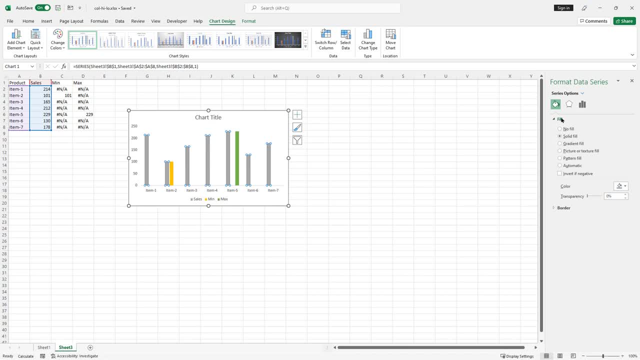 Now I can mush them all together. Basically they're going to overlap. Go into my series options here where it says series overlap. Bring that all the way to 100%. You can see now they've all combined over each other. I don't need this label anymore. Click that.